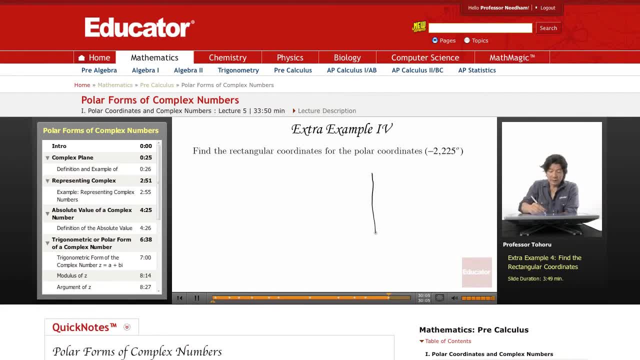 One final example here. Let's draw our grid again. Okay, here we have negative 2. This is an interesting one. So 225, where is that? Okay, now, a couple ways you can look at it. You can say, okay, well, I just like to start. okay, well, 280, right, Or 180, rather right, And so you kind of figure: okay, you know what's there and what's left. So we kind of go 225 minus 180, right, And then we go 5, right, 4, 45 degrees. 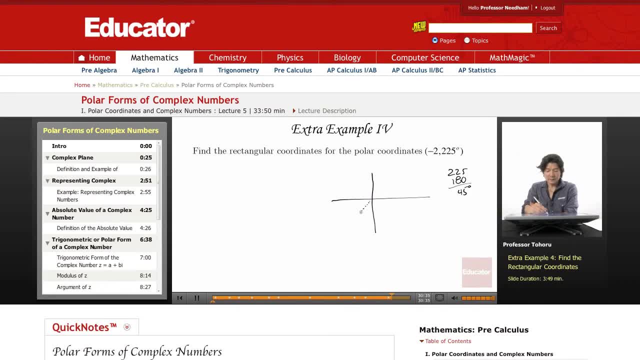 So we know it's going to end up down here, right? I'm just going to put it down here, right? So this is the angle that we end up with, right, Theta equals. the reference angle is 45, right, It's roughly 45. However, what is it? It's negative 2.. So where is it going to be? It's going to be out here, right? So this is actually where it's going to end up. So this is actually the point: negative 2, 225, right. 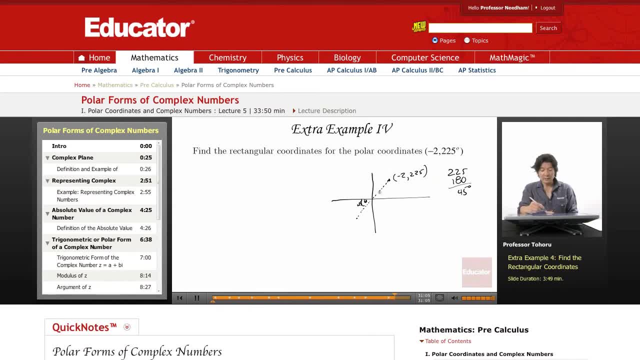 Weird, right, But the idea is that with polar coordinates, you follow the angle. If it's negative, you have to go in the opposite direction and find your new angle, okay. So what I would do in this case is for theta find out what this new angle is- 45, and you know you're up in this quadrant. okay, So let's think about this. So you know that this is 2,. okay, So what I would do is I would say: okay, since we have a 45, 45 triangle, right, We know that this is 2,, this is. 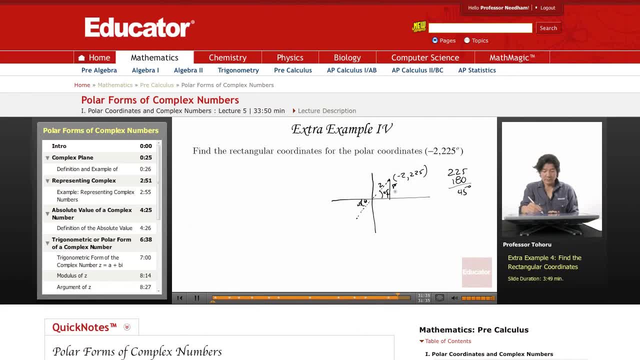 going to have to be what 2 divided by root 2.. So I'm going to call this: why don't we do this? So we know that the x point from here to here right is going to have to be: yeah, let's do it this way: r cosine theta. Let's do it this way, right r. in this case, this is 2, cosine theta. What's?